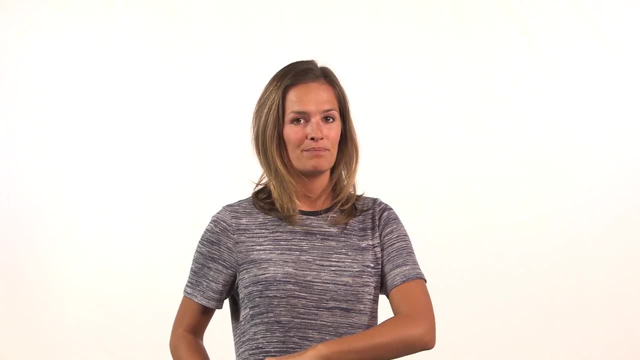 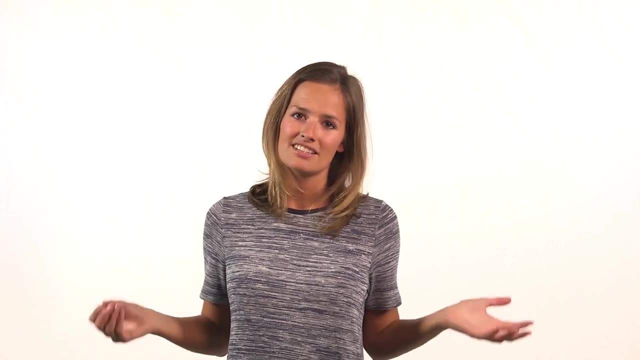 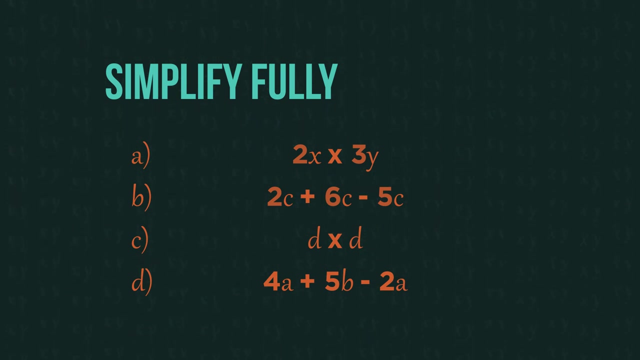 letters, so this is the simplest form. This expression might represent eight apples and two bananas, which are completely different things. so we can't combine them, Can you? When you simplify these four things, don't worry, if you aren't sure, just give them. 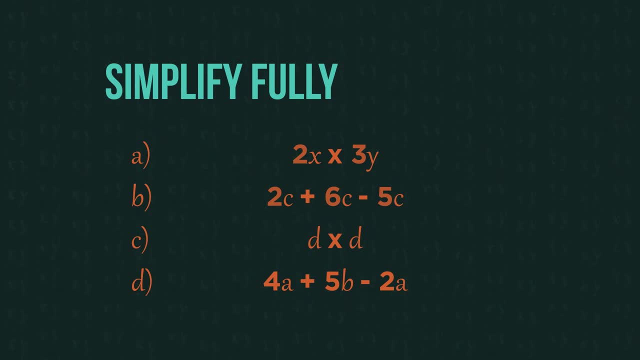 a go and we'll go through the explanations after. Pause the video, try the questions and click play when you're ready. How did you get on For the first one we just do: 2 multiplied by 3 is 6 and remove the multiplication sign. 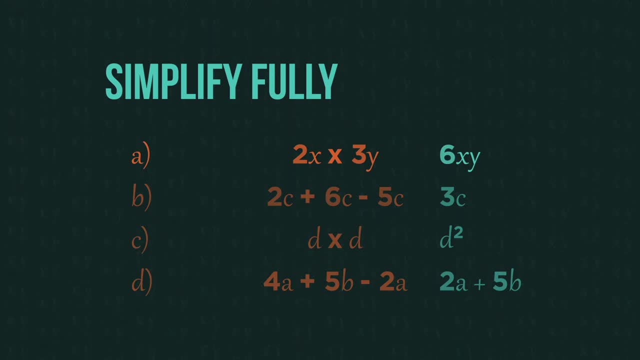 so we get 6xy. In the second one we group the same letters together. so 2 plus 6 minus 5 gives us 3c. Here we need to get rid of the multiplication sign, which would give us dd. but we can improve. 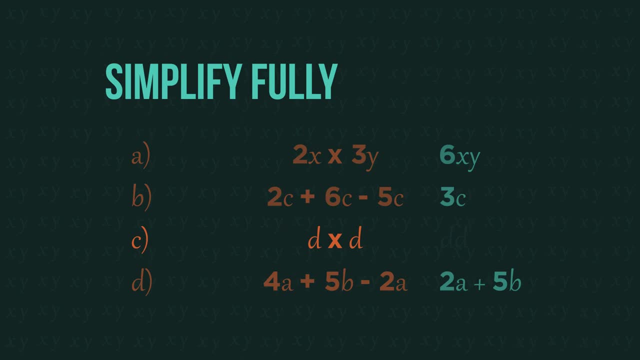 on that even further by writing d squared. If the question had been this, then it would be: d cubed Subtitles by the Amaraorg community. All this would be d to the power of 4.. And then, similar to the second question, we group the same letters together, but they: 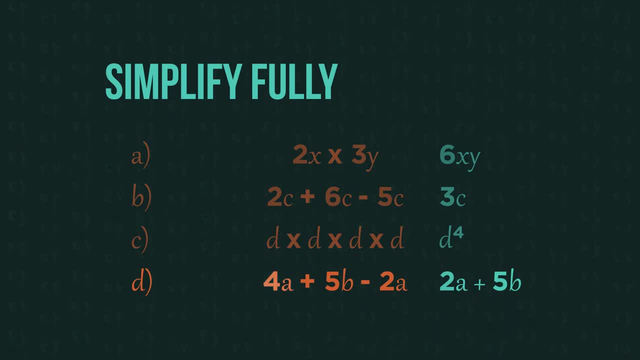 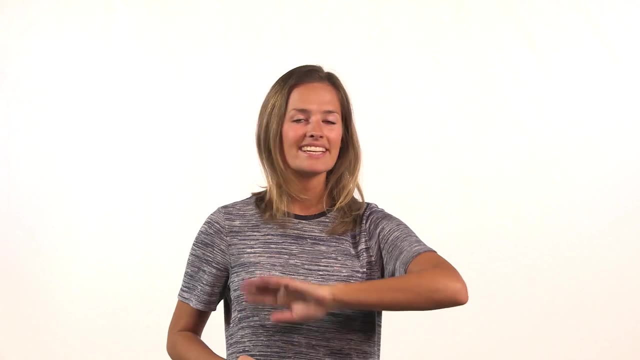 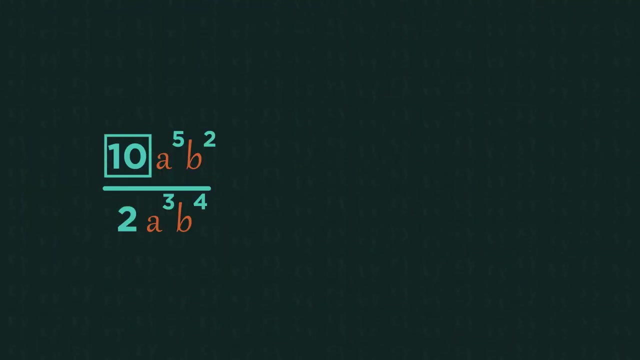 must be the same letter. so 4a subtract 2a is 2a For division. you can cancel out the numbers exactly as you would with fractions, and we can also cancel out letters. so 10 divided by 2 is 5.. 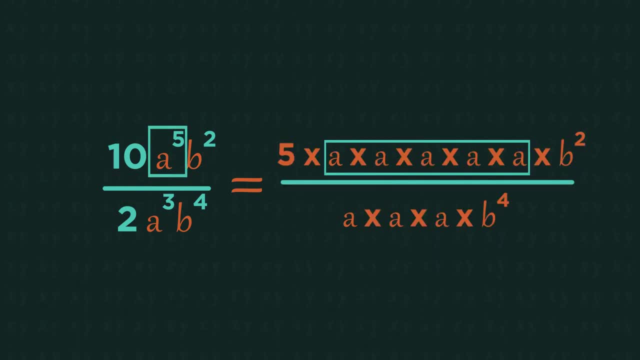 And then, because we have 5a's in the numerator and there are 3 in the denominator, this means we can cancel out 3 of the a's from both the numerator and denominator, leaving just 2a's in the numerator. 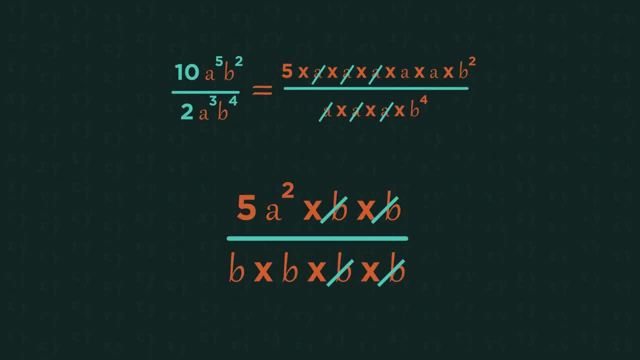 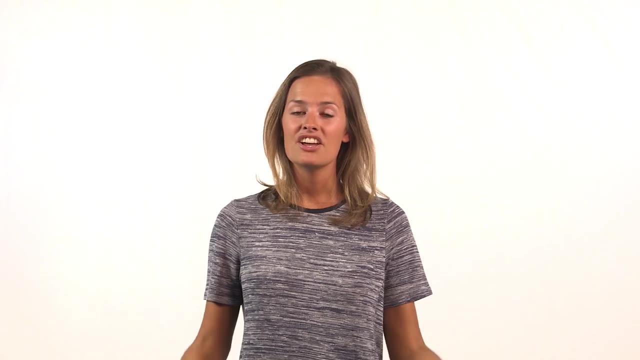 And then the same for the b's: We can cancel out 2b's, leaving just 2b's in the denominator, giving us our final answer. Subtitles by the Amaraorg community. Subtitles by the Amaraorg community. Subtitles by the Amaraorg community. 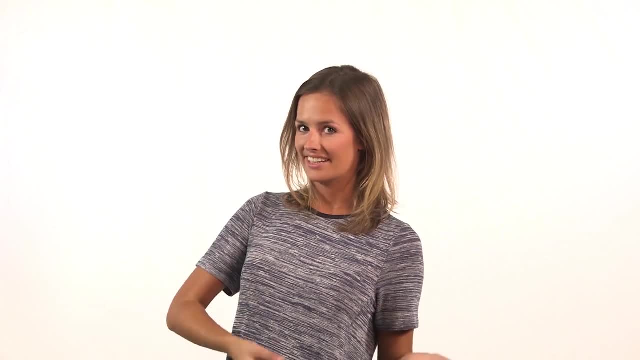